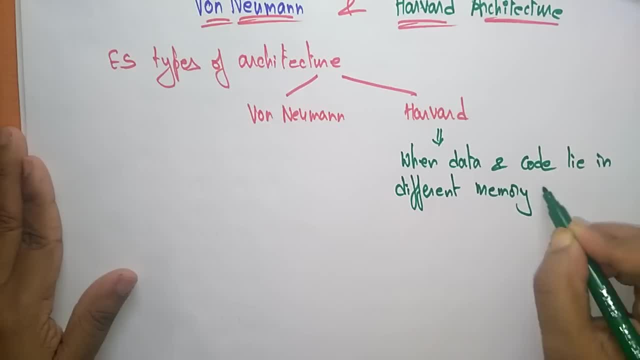 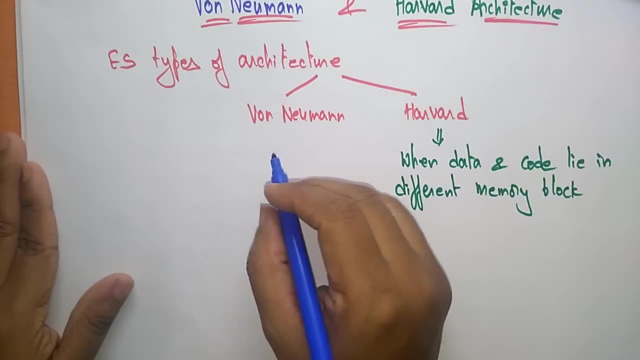 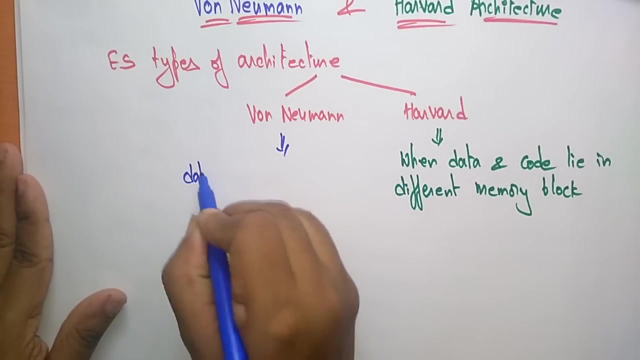 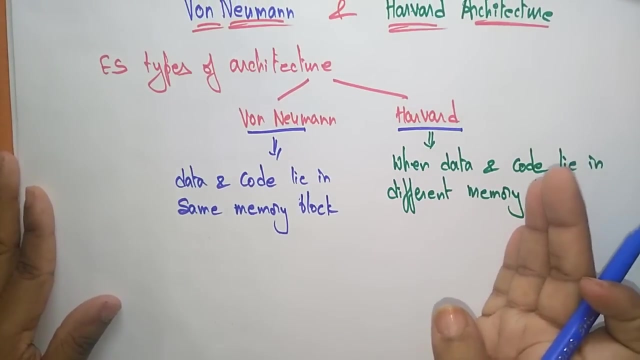 this point, different memory block That referred as a hardware architecture. okay, So whereas in von Neumann architecture data and code lie in same memory block, Data and code lie in same memory block. So that is the main difference between the von Neumann and the hardware In the hardware architecture. 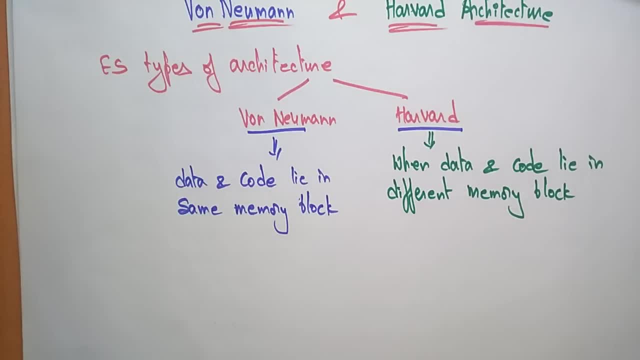 complete, whatever the data that we are using and whatever the built in code that is there. so means the data and the instruction. Data memory and instruction memory lie in different memory blocks. they are separate memory blocks, Whereas in von Neumann architecture you have to stay in the statement, you have to interact with your students and the человека. So data management is superficial and functional, Living the in cord. it is only shown in code. There doesn't need center etc and etc in advanced instruction module. But rich or poor understanding, we didn't use it in ever. So we have a educational episode we can come back here. Goodbye. 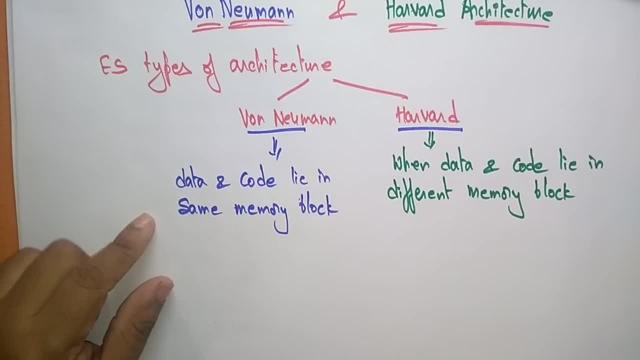 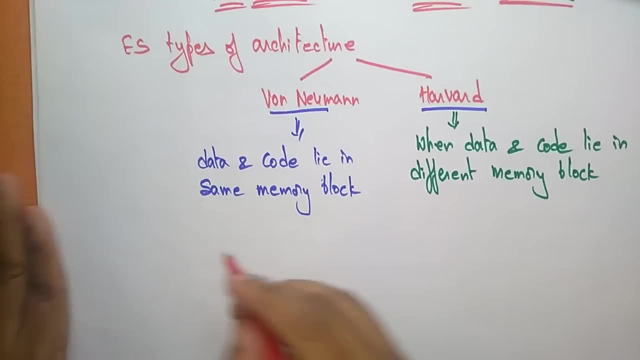 both the data and the instructions will be stored in the same memory block. so that's the main difference between von Neumann and hardware. so let me explain about exactly what von Neumann architecture consists of. von Neumann architecture. so in this architecture, one data path or one bus. 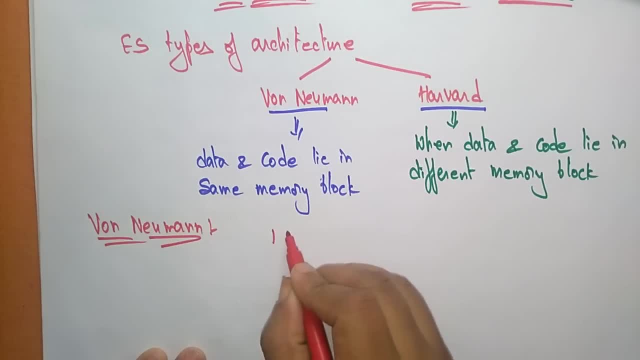 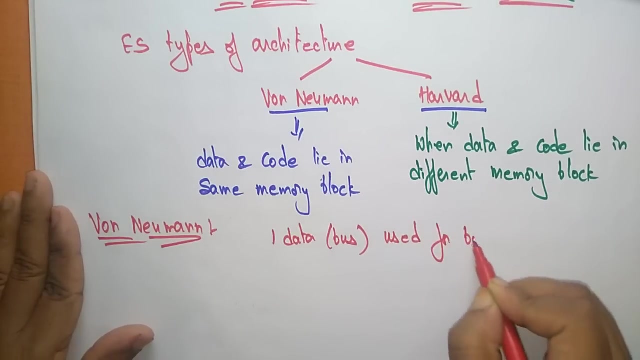 exists for both instruction and data. suppose, whatever the data path, that is there data, or you can take it as a bus, whether that bus is an address bus, data bus or control bus, so that bus, only one bus, is used for, used for both instructions and the data. 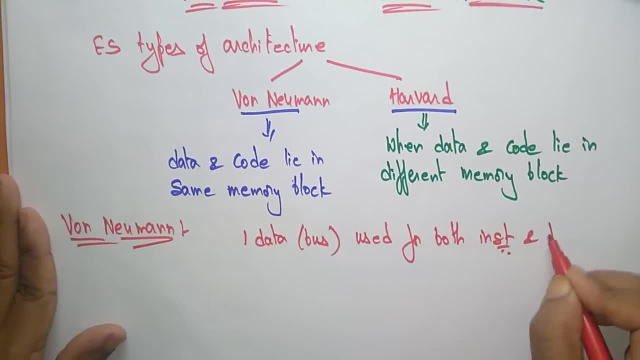 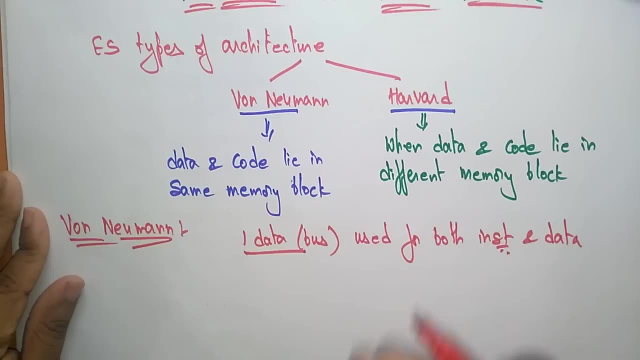 means both used for the code as well as the data. so only one data bus is used for both instructions and data. so, as a result, CPU does one operation at a time. so by doing this, CPU can, can, can, can, can perform only one operation at a time. one operation at a time, so that is either fetching of data or 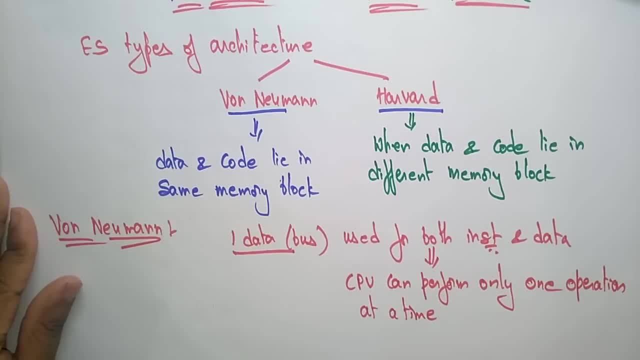 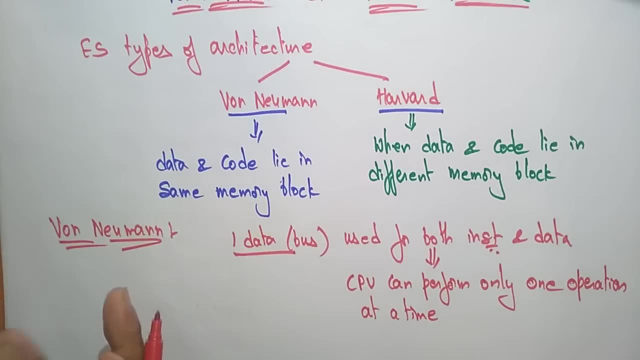 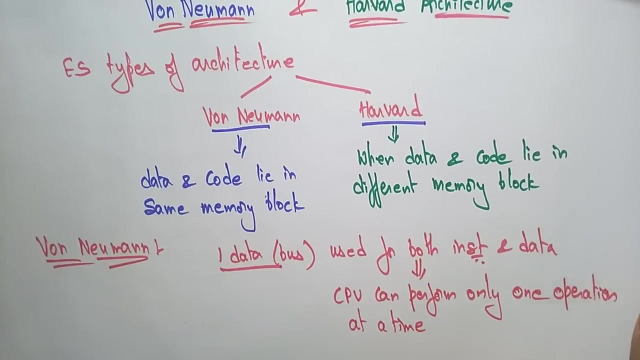 instruction from memory or performing read, write operations on data. anything, any one operation can be done at a time. so that is the von Neumann architecture. so it means it allows only the single and sequential memory. this von Neumann architecture allows use of single and sequential memory. so when it supports only the simple hardware, why it is only support simple hardware? 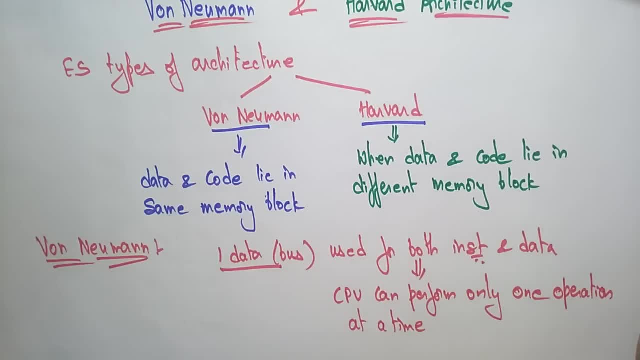 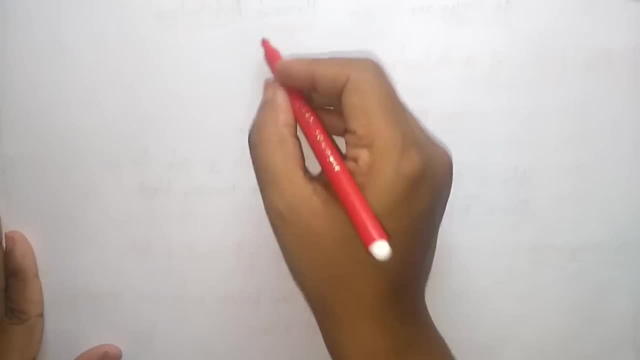 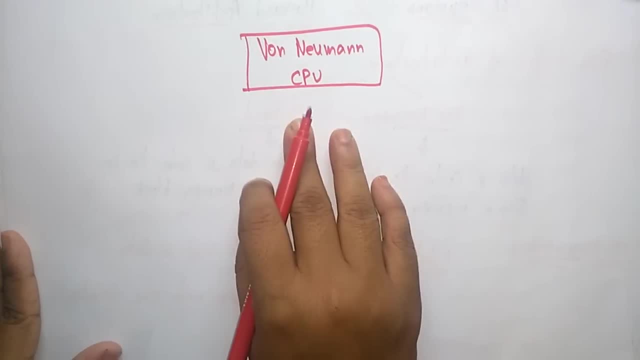 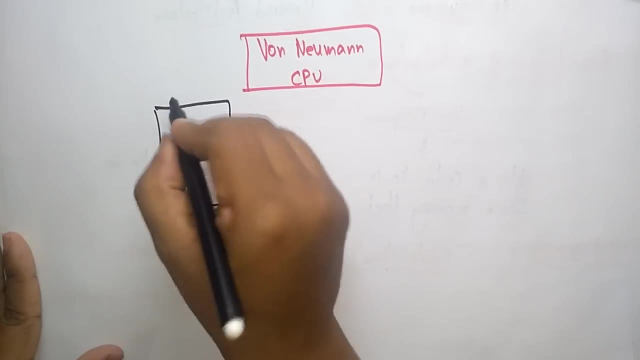 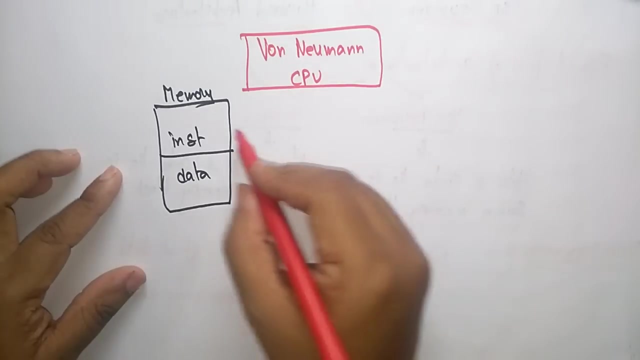 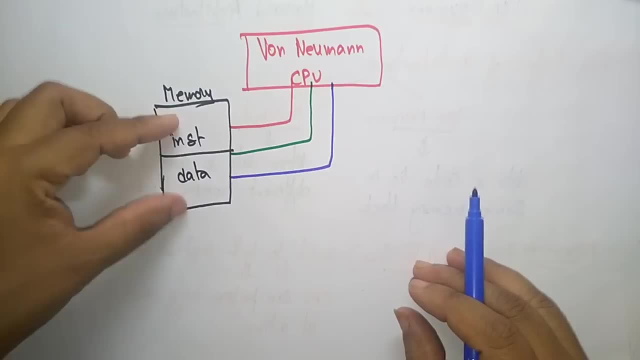 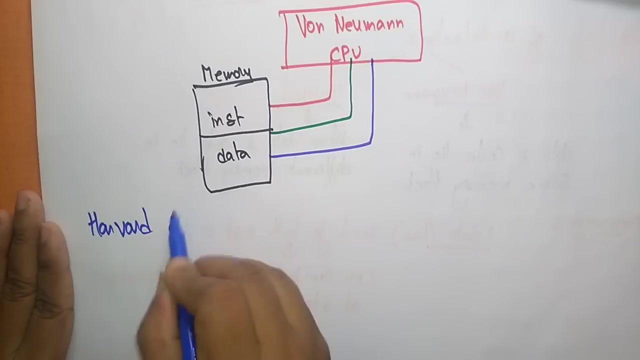 so? So all this address bus, data bus and control bus is accessing only one memory block, that you call it as a Von Neumann architecture. So now let me explain about the hardware architecture. Hardware architecture. So what is this hardware architecture? 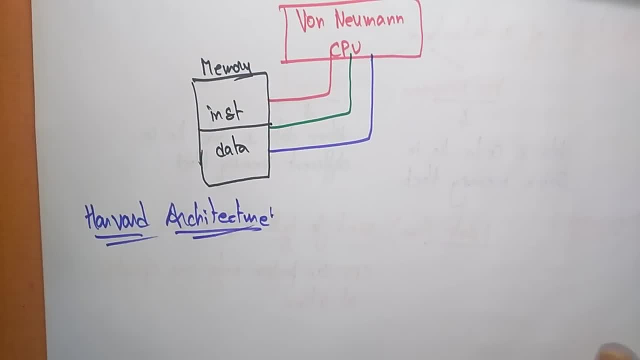 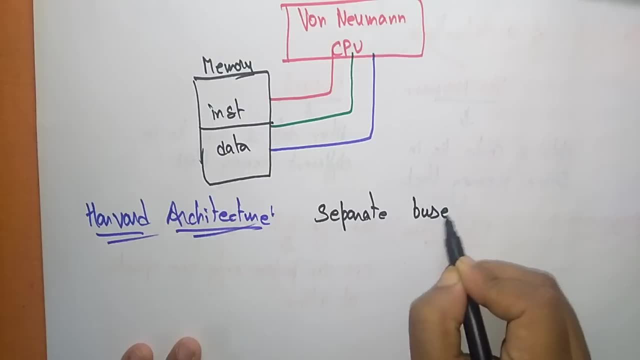 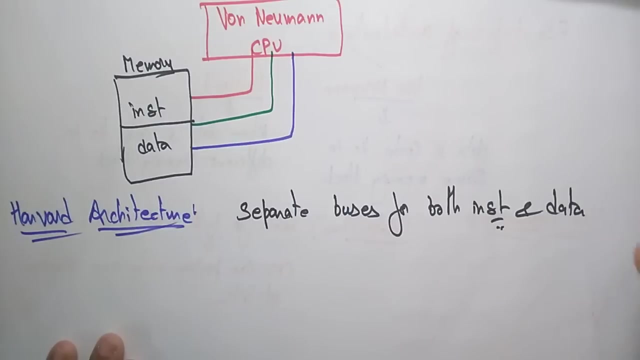 It offers separate storage and signal buses for instructions and data, So it's just using separate buses for both instruction as well as data. So data can be accessed by one bus and instruction memory can be accessed by another bus. So this architecture has data storage entirely contained within the CPU. 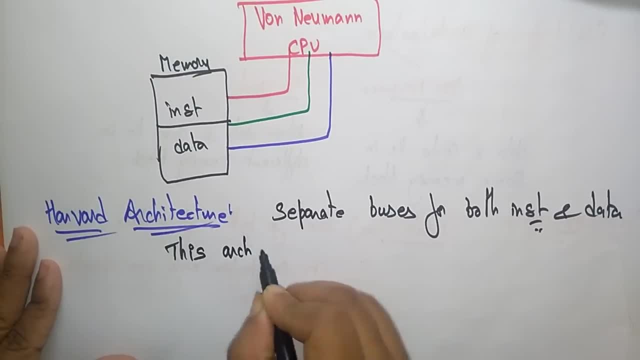 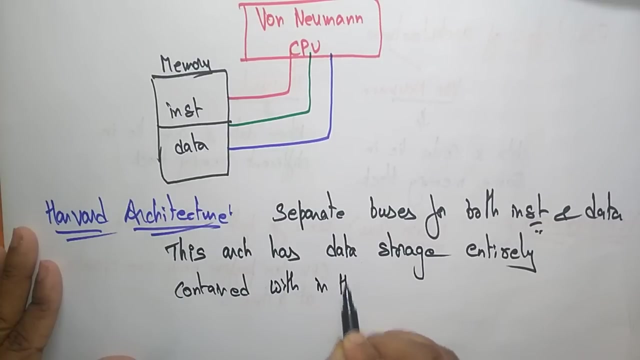 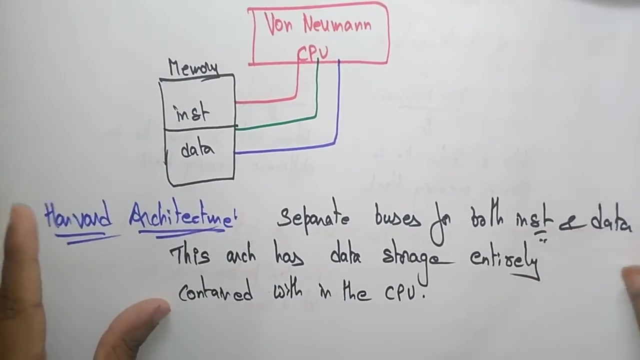 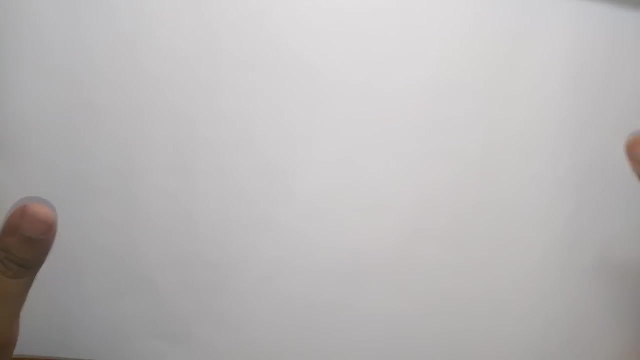 This architecture has data storage- So remember this point- within the CPU. So here the computers have separate memory area for data as well as a program instruction, So both the data and the program instructions- using internal data buses, So which is allowing simultaneous access for both data and instructions. 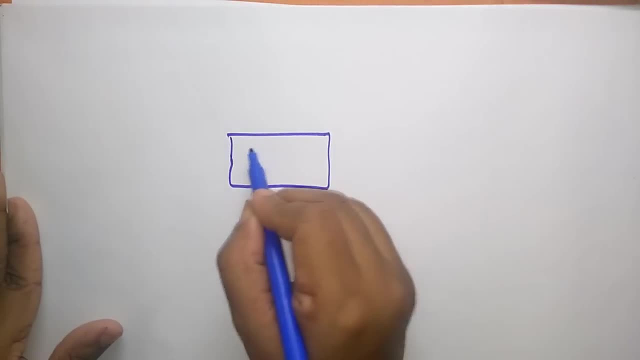 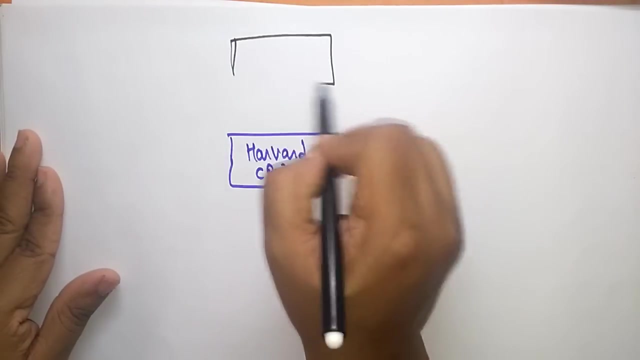 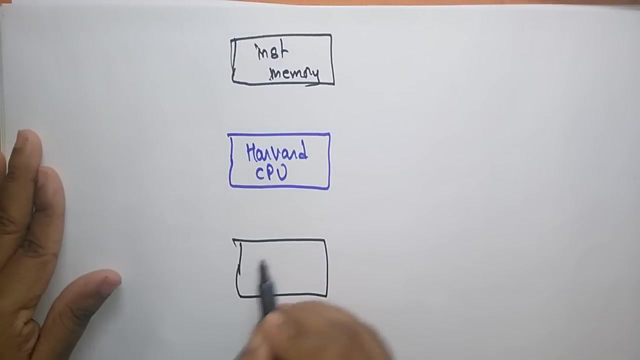 So let me show you. This is a hardware. This is a hardware CPU. This hardware CPU is having the separate memory blocks: One is for instruction memory- Instruction memory- And another is for data memory- Data memory. Okay, So each is having the separate buses. 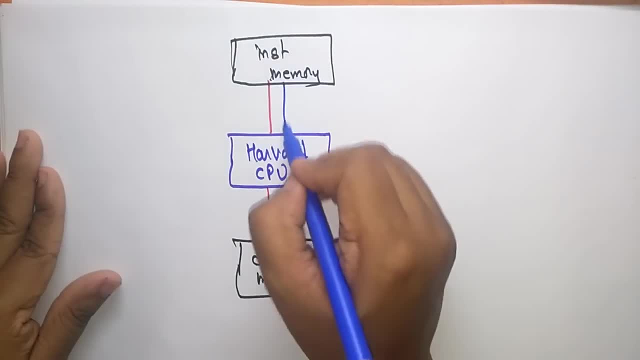 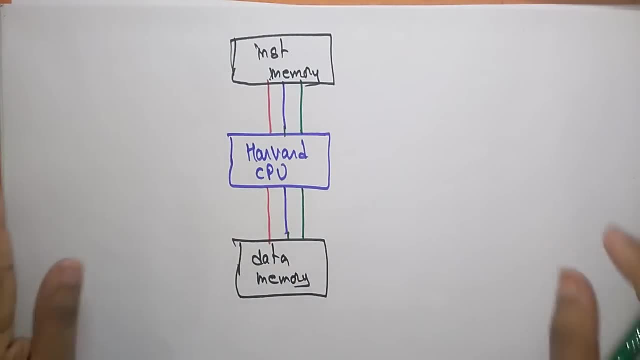 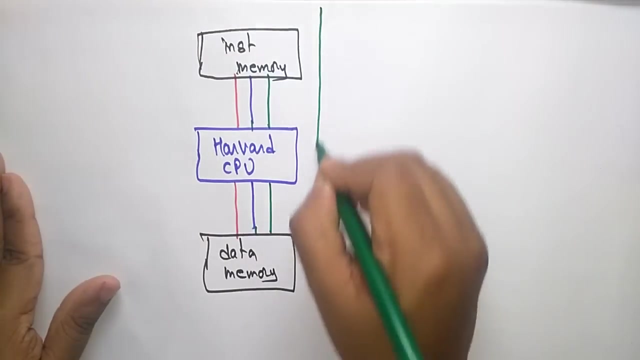 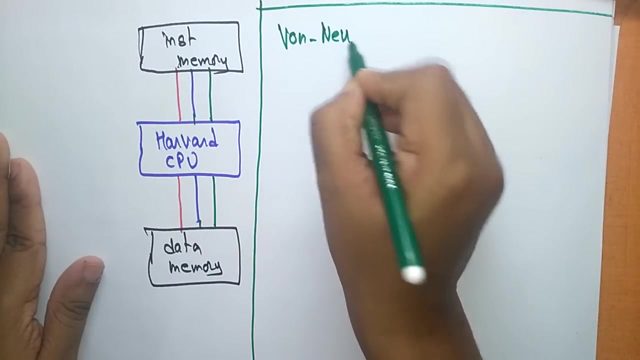 That is, the address bus, data bus, as well as the control bus, So each having the separate buses. So this is about the hardware architecture. So let me explain you the difference between the hardware and the Von Neumann: Von Neumann architecture and hardware architecture. 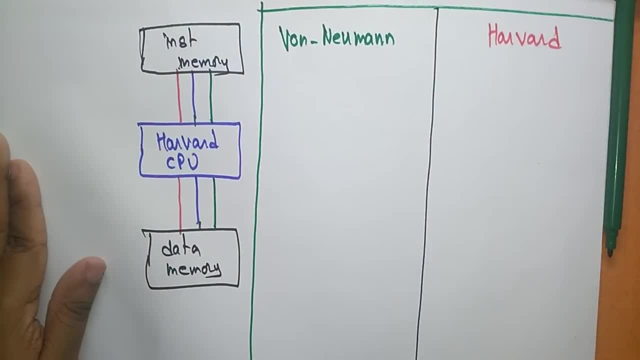 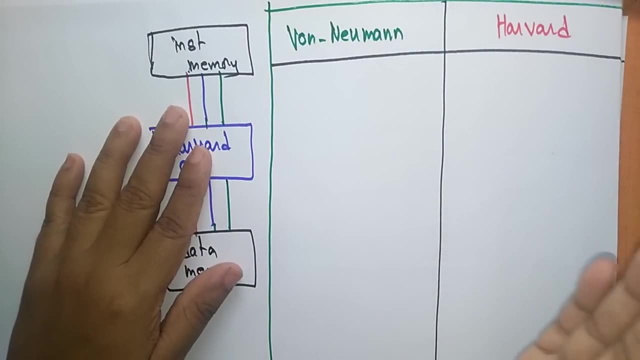 So let me explain you the difference between these, both Von Neumann and the hardware architecture. Okay, So what I said? Von Neumann is using only the single memory, and that single memory has to be shared by both code as well as the data. 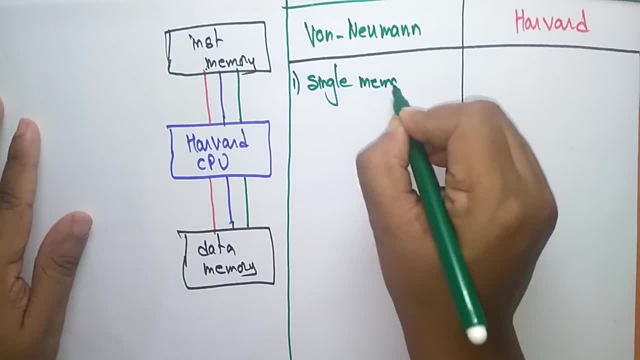 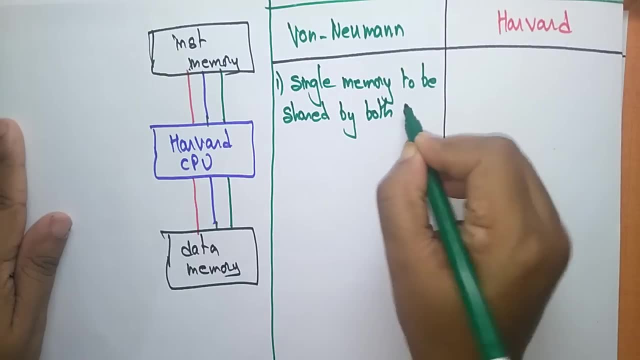 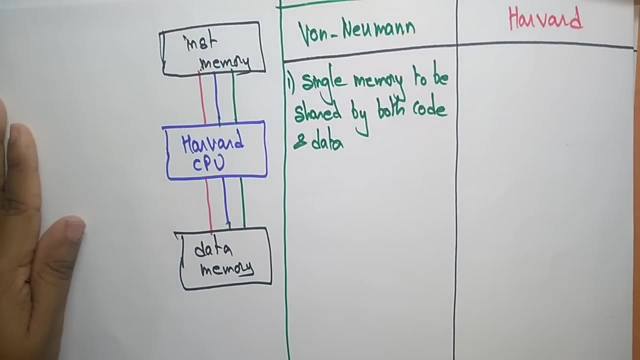 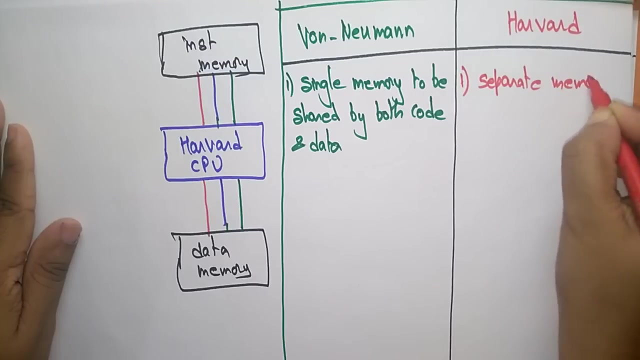 So single memory to be shared by both code and data. That is the instruction, and the data will be shared only with the help of the single bus. Where is the hardware? Hardware uses the separate memories for both for code and data. And next point: 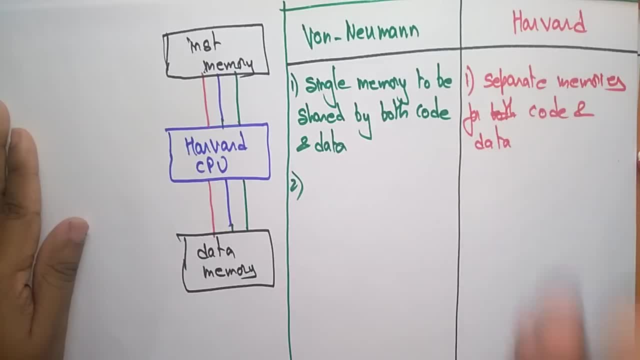 So Von Neumann architecture. here the processor has to fetch code in one clock cycle and data in another clock cycle. So it requires two set of clock cycles. Two set of Clock cycles required in Von Neumann architecture, So one cycle for data fetch and another cycle for instruction fetch. 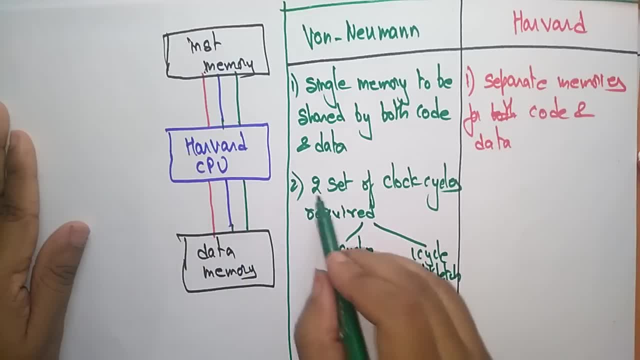 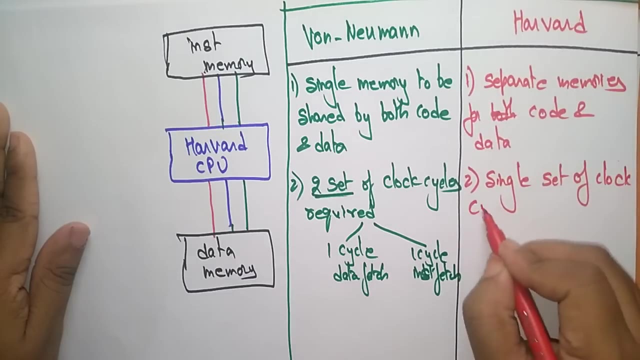 Instruction fetch. So total, it requires two set of clock cycles. So whereas in Von Neumann hardware architecture single set of clock cycle is sufficient, Single set of clock cycle is sufficient. Why single cycle of clock cycle is sufficient? Because as separate buses are used to access the code and data. 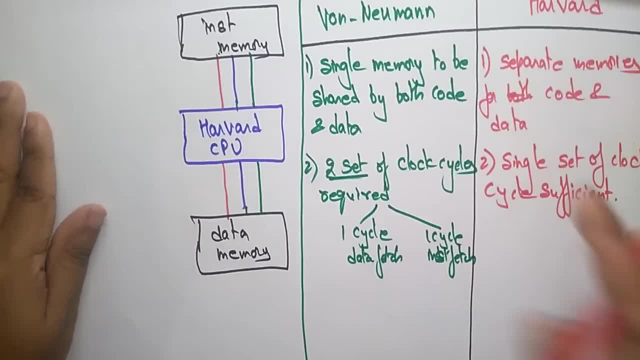 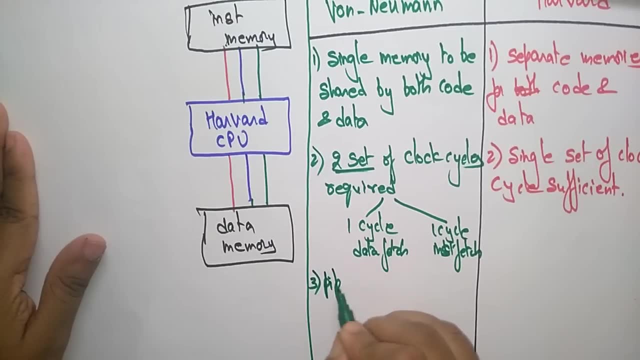 So single set is enough. And next is here: in Von Neumann architecture, pipelining is not possible. Pipelining, Pipelining, Pipelining, Pipelining, Pipelining, Pipelining, Pipelining.